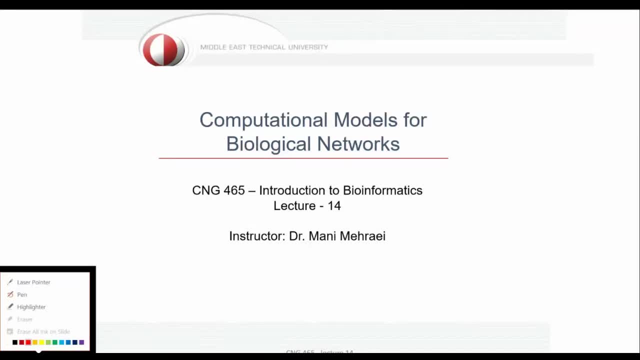 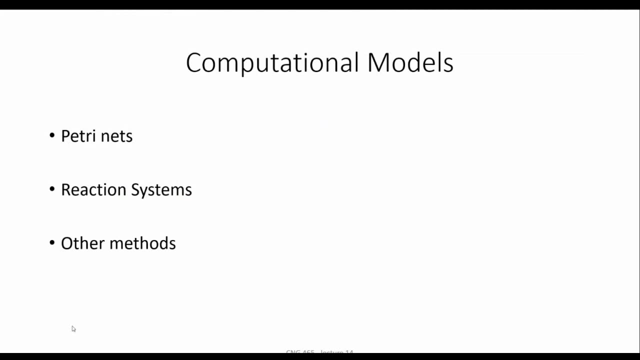 with such biological systems. Fortunately, I think, now the slides are loaded, so you can see the slides. Let's test it. I hope there's no problem with viewing the slides now. Okay, so there are several methods to deal with that, as I said, PetriNet and Reaction Systems. 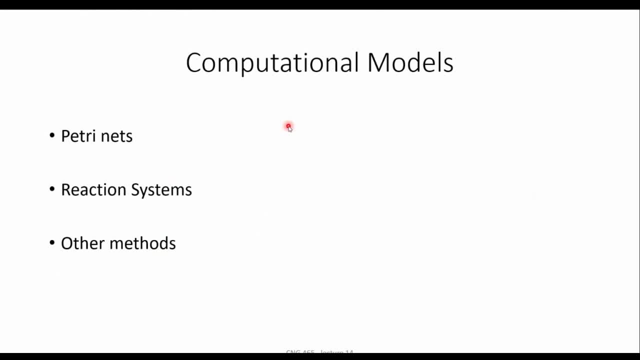 personally, I worked with them. That's why I chose these two. Otherwise it's not. I cannot claim for tex them. that's why I chose these two, Otherwise it's not. I cannot claim for are the best ones, but it depends on the biological system that you are modeling. 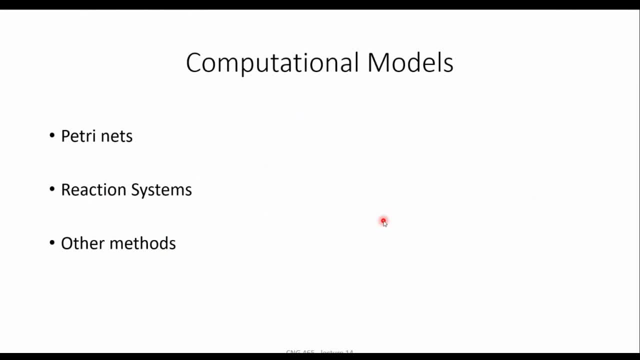 with, and now I talk about the challenges we have for computational models and also what are the advantage of them. so let's give an example related to biological network like this one. this image is related to hemoglobin switching. so a hemoglobin goes through changes. it means that there are some gene. 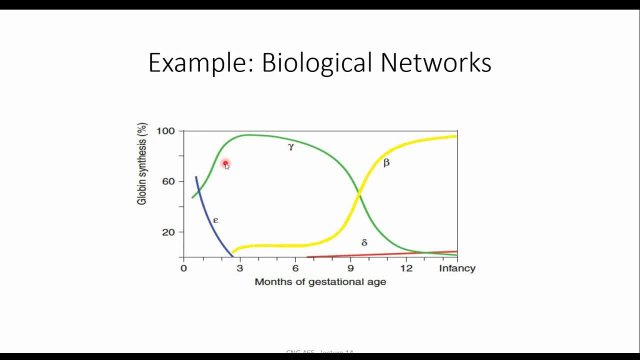 expressions which are upregulated and down regulated through time. this part, until unit 3, is related to embryonic stage, from 3 to 9 or even we could say 12. we are dealing with fetal stage and starting from stage 3 to stage 5.. 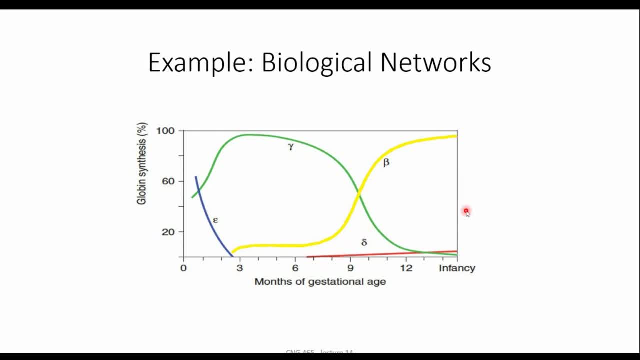 from 9 until the person is alive. so we are dealing with adults hemoglobin. now, as you can see, the level of gene expressions are changing through time, like, for example, gamma is up regulated during the fetal life, but it starts to be down regulated in the adult life. so that's why we call it a switching and as 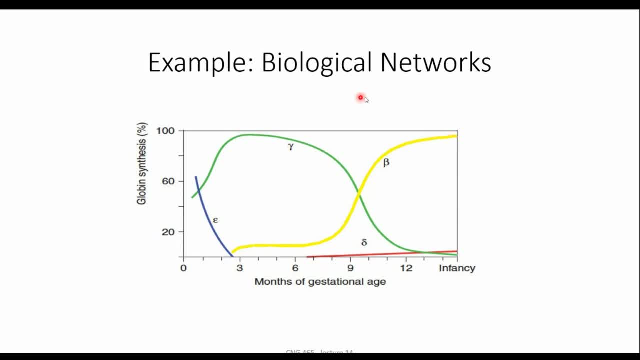 you can see, for beta this is a different story, and hemoglobin also deals with alpha, which is not included in this picture. also, there might be other genes involved with it, but usually we try to simplify everything in order to have easier time for modeling. but you may say, if we neglect some, 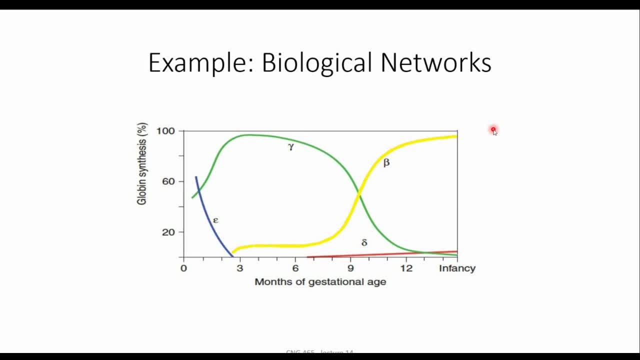 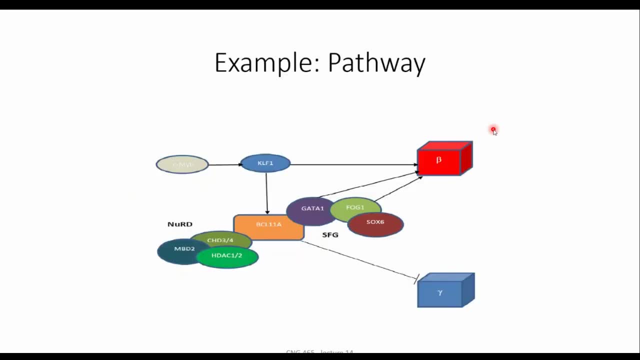 important genes, then we don't have time to model it and we don't have time to model it and we don't have time to model it and we don't have time to factors. what will happen? would it be natural? would it give us the correct model? yes, these are the challenges that we are facing in computational modeling. 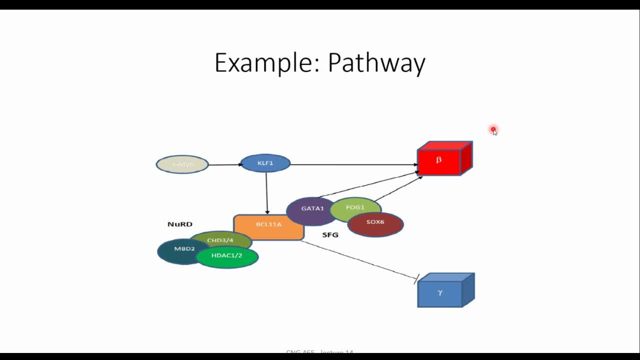 so we try to include components which are involved in it as much as possible. now, based on the pathways, we can design our model. so this is a pathway. and based on the articles that we are reading from other reasons, we can design our model. so this is a pathway and based on the articles that we are reading from other reasons. 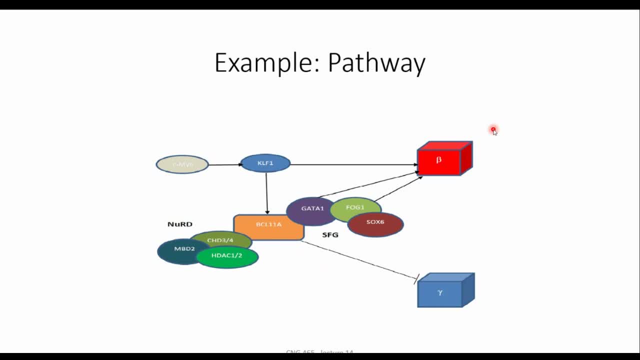 we can design our model. so this is a pathway and based on the articles that we are reading from other reasons- researchers- maybe we understand that there should be more to it. for example, researchers: maybe we understand that there should be more to it. for example, researchers: maybe we understand that there should be more to it. for example, when you find a pathway inside cake. 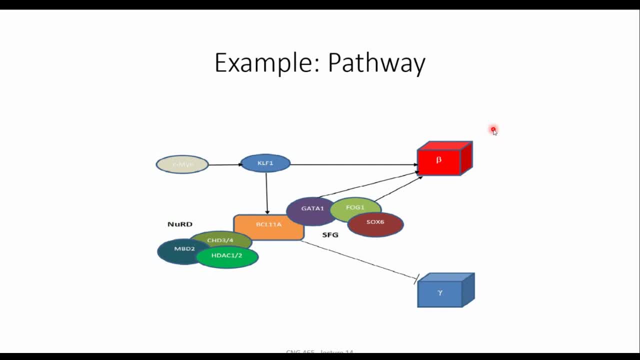 when you find a pathway inside cake. when you find a pathway inside cake website- maybe there are more components website. maybe there are more components website. maybe there are more components involved- then you can add it to your involved. then you can add it to your involved. then you can add it to your pathways. okay, because this is your model. 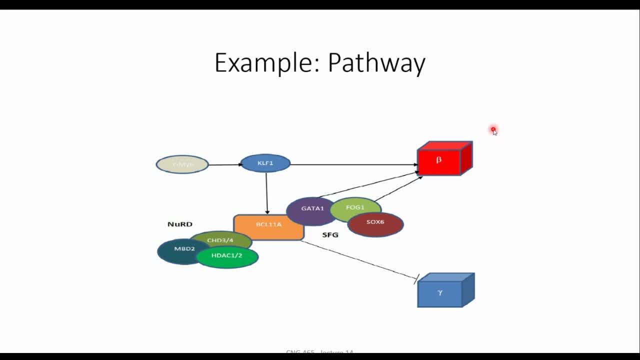 pathways- okay, because this is your model. pathways- okay, because this is your model, and then you should show that this is, and then you should show that this is, and then you should show that this is working properly and you should validate working properly and you should validate working properly and you should validate that. so, for beta-globin and gamma, 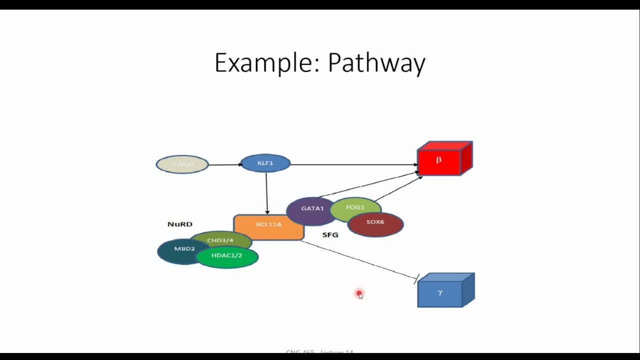 that so for beta-globin and gamma. that so for beta-globin and gamma globin in this hemoglobin switching globin in this hemoglobin switching globin in this hemoglobin switching network. you can see that you have such a network. you can see that you have such a. 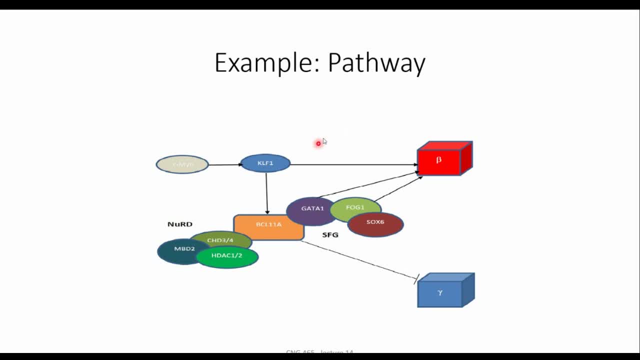 network. you can see that you have such a pathway. there are some proteins and pathway. there are some proteins and pathway. there are some proteins and components involving this, for example, components involving this. for example, components involving this. for example, you know that klf1 is upregulated engine. 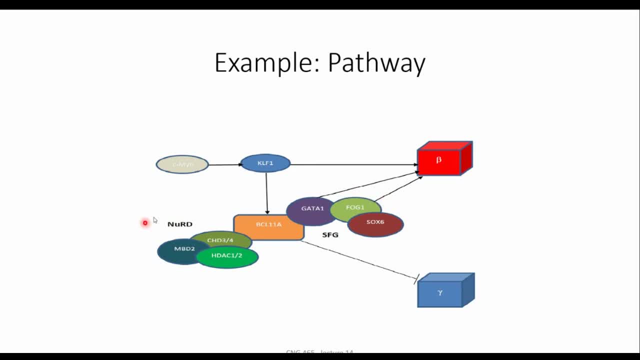 you know that klf1 is upregulated engine. you know that klf1 is upregulated engine. the gene expression of beta, and this the gene expression of beta, and this the gene expression of beta. and this multi complex protein, this one multi complex protein, this one. 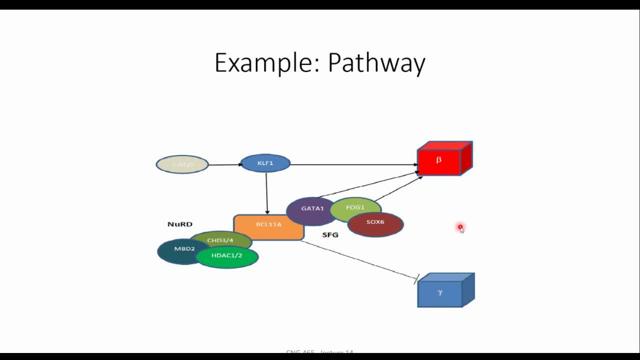 multi complex protein. this one inhibits gamma expression and that's the inhibits gamma expression and that's the inhibits gamma expression and that's the reason. in this picture you can see gamma reason. in this picture you can see gamma reason. in this picture you can see gamma is down regulating after time and beta. 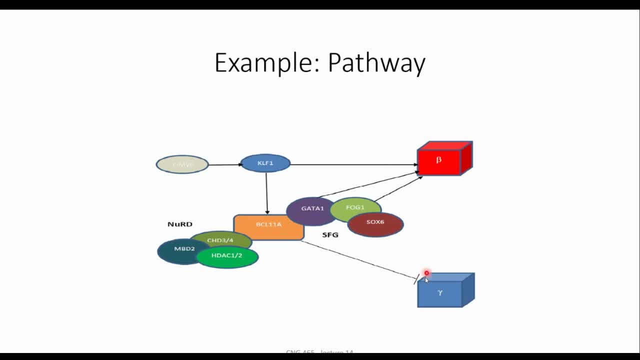 is down regulating after time and beta is down regulating after time and beta is up regulated. so, as you can see, by is up regulated. so, as you can see, by is up regulated. so, as you can see, by using such pathways, you can show what's. using such pathways, you can show what's. 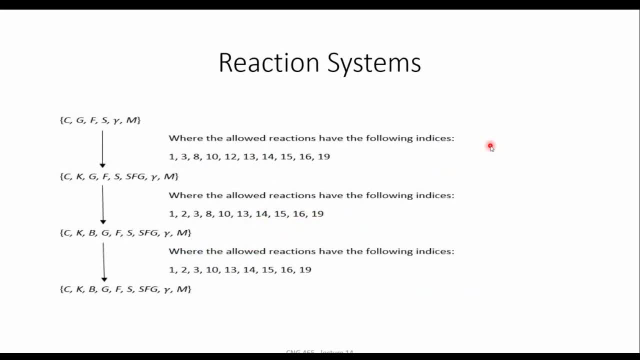 using such pathways, you can show what's going on in details in terms of going on in details, in terms of going on in details in terms of biological networks. now we can use biological networks. now we can use biological networks. now we can use different computational methods. one of 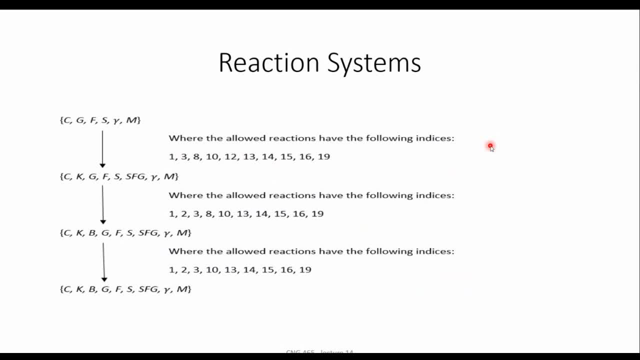 different computational methods. one of different computational methods. one of them is reaction systems. reaction them is reaction systems. reaction systems could be useful for, just as systems could be useful for, just as systems could be useful for just as. specifying that, whether a protein level, specifying that, whether a protein level. 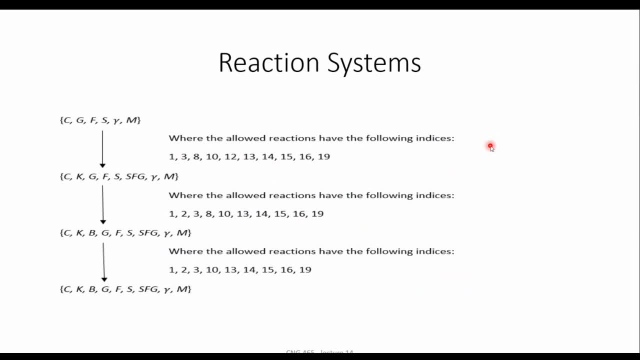 specifying that, whether a protein level or, for example, mRNA level is high or low, or, for example, mRNA level is high or low, or, for example, mRNA level is high or low, or, for example, if the gene expression is, or, for example, if the gene expression is, or, for example, if the gene expression is up regulated or down regulated, like by: 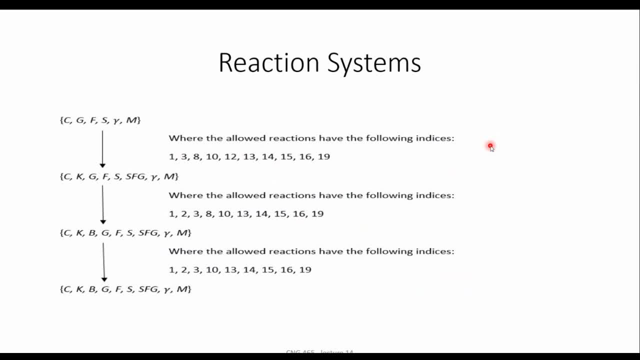 up regulated or down regulated, like by. up regulated or down regulated, like by showing the components of inputs, outputs. showing the components of inputs, outputs. showing the components of inputs, outputs and inhibition, for example, in the, and. inhibition, for example in the, and inhibition, for example, in the previous picture. 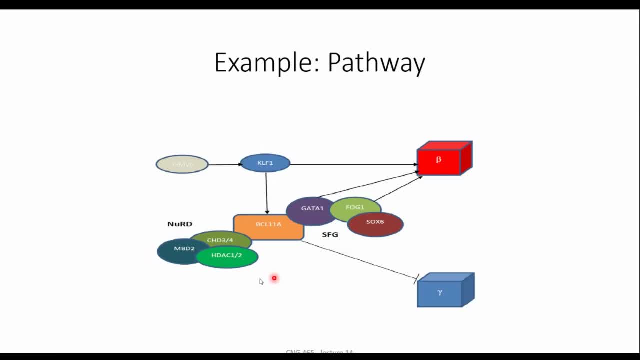 previous picture. previous picture: this part, this part, this part is inhibition. so when you have such a is inhibition. so when you have such a is inhibition, so when you have such a multi-complex protein, whenever you have multi-complex protein, whenever you have multi-complex protein, whenever you have it as input, then you should know that it. 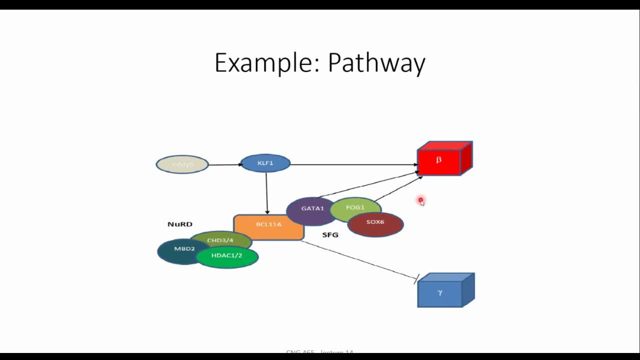 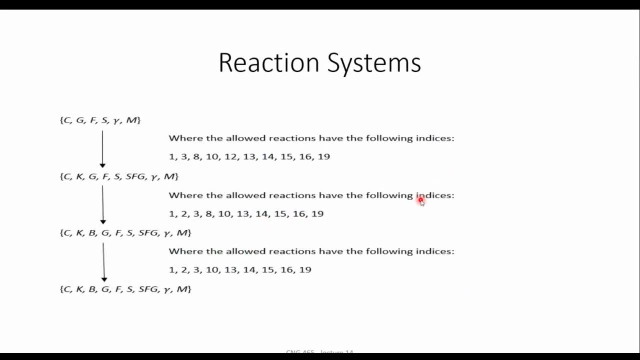 it as input, then you should know that it it as input, then you should know that it inhibits, for example gamma gene inhibits, for example gamma gene inhibits, for example gamma gene expression. so by using those two, three expression, so by using those two, three expression, so by using those two, three components, you can specify exactly. 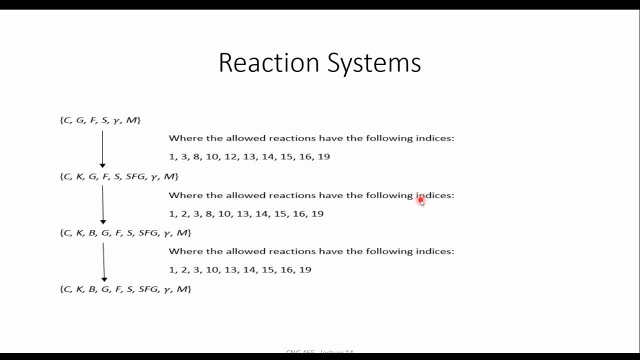 components. you can specify exactly components. you can specify exactly what's going on in the state of in terms. what's going on in the state of in terms? what's going on in the state of in terms of biological networks? what's the of biological networks? what's the? 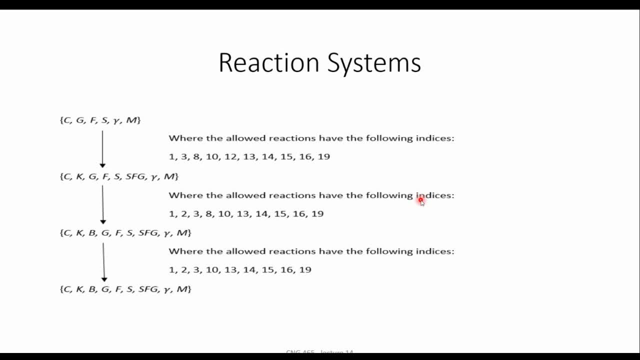 of biological networks. what's the disadvantage of that? the thing is that disadvantage of that. the thing is that disadvantage of that. the thing is that i'm interested to know what is exactly. i'm interested to know what is exactly. i'm interested to know what is exactly the level. 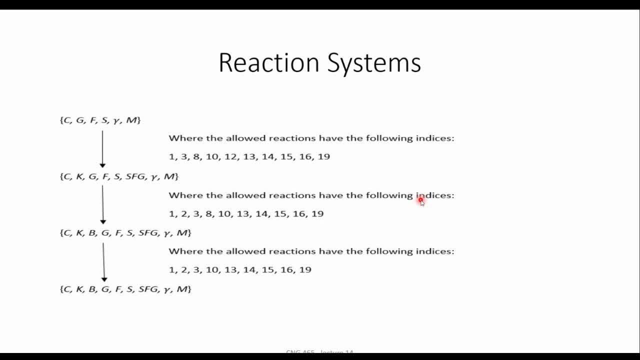 the level. the level, or even not exactly, well approximately, or even not exactly well approximately, or even not exactly well approximately. what's the level of the mrna that i'm? what's the level of the mrna that i'm? what's the level of the mrna that i'm looking for? 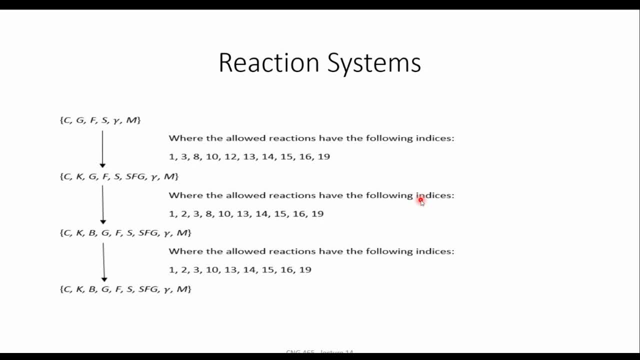 looking for, looking for how much of beta chain i will have, at how much of beta chain i will have, at how much of beta chain i will have at the end, the end, the end, this type of questions, unfortunately, this type of questions. unfortunately, this type of questions, unfortunately, reaction systems. 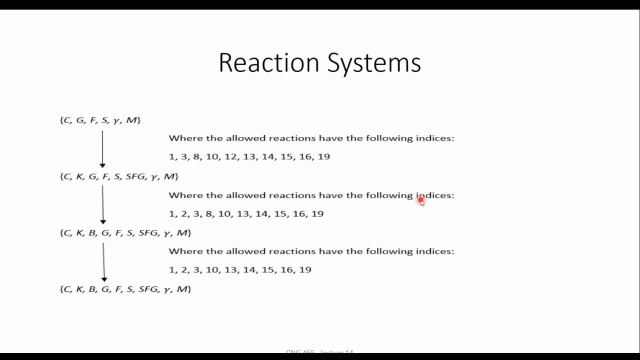 reaction systems. reaction systems cannot answer, and that's a big cannot answer, and that's a big cannot answer, and that's a big disadvantage of that, disadvantage of that, disadvantage of that. so this one can be useful, as i said to. so this one can be useful, as i said to. 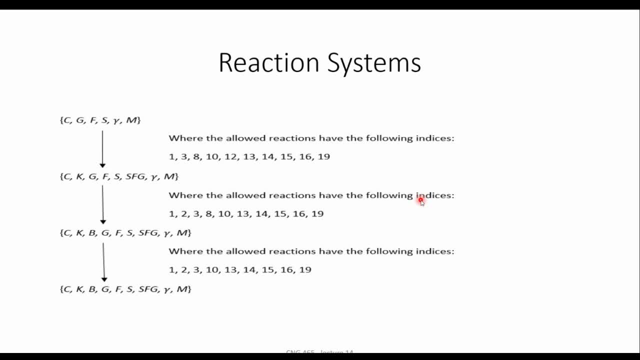 so this one can be useful, as i said, to just know, just know, just know whether at the end we will have, whether at the end we will have, whether at the end we will have some, for example, gamma chain or beta, some, for example, gamma chain or beta. 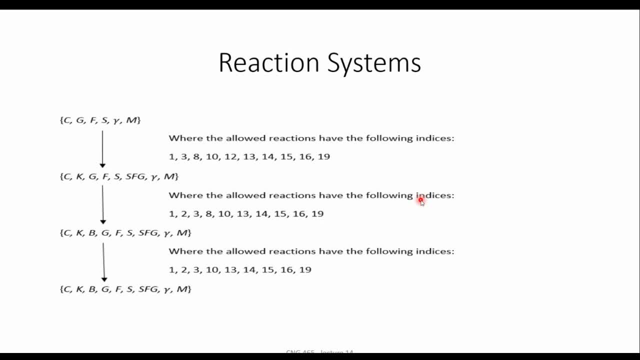 some, for example, gamma chain or beta chain, or chain or chain, or this is totally uh, knocked down. this is totally uh, knocked down. this is totally uh knocked down. that's why we can predict things using. that's why we can predict things using. that's why we can predict things using reaction system. 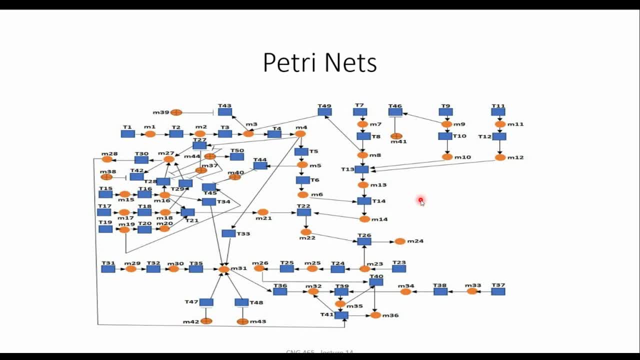 reaction system: reaction system, but there are other computational methods. but there are other computational methods. but there are other computational methods like like patronet, as a directed graph mathematical method. this one can be very useful because this is very flexible and we can add different properties to it, and by using that, 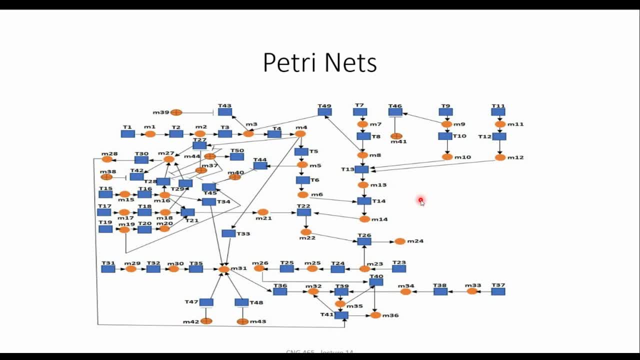 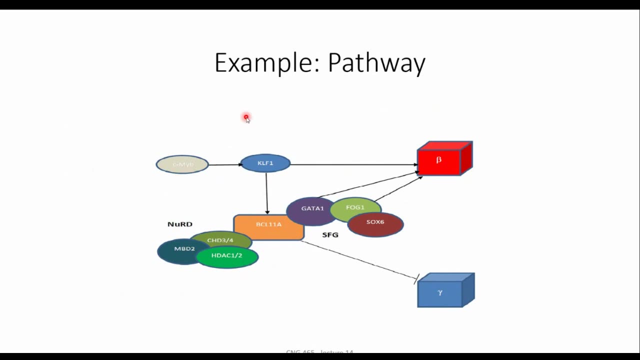 you can even understand approximately what would be the level, for example, for beta globing. so this patchnet that you can see here is derived from this pathway. so it takes time to be to get yourself familiar with how you can model everything in terms of patronet, but as soon as 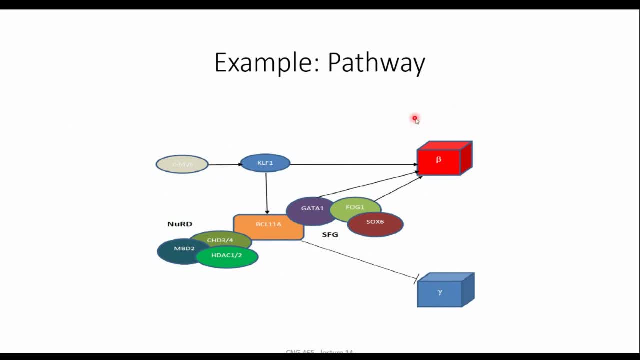 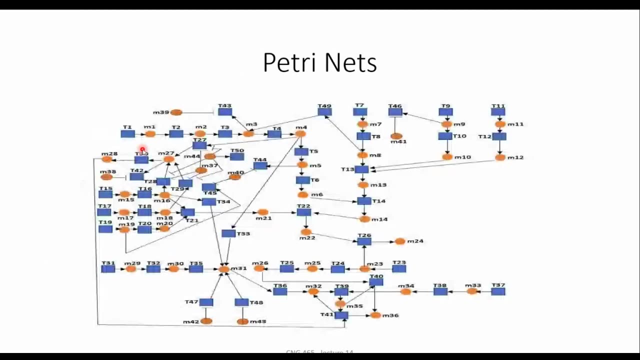 you do, things will be much easier for you to deal with that. but before that we should know about the properties related to patronet. so the classical one is a discrete patronet. it means that here in this picture you have places and transitions, these uh, circle ones. there are places, they can denote the entities, like, for example, mrna. 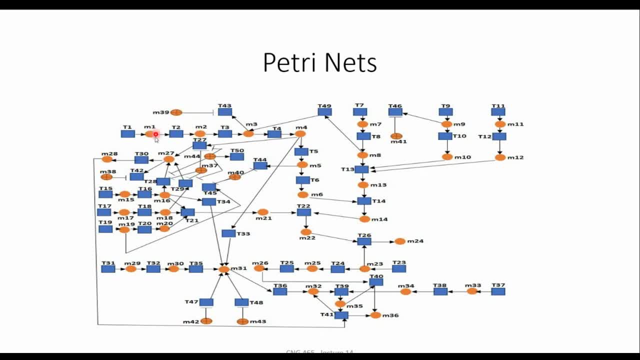 genes, protein, so these circles can identify them, even mutations, even for in terms of mutations, you can show it by using places. transitions are the actions happening in biological systems, like two entities are binding together, for example, or many proteins are binding together to have a complex multi-protein. so these transitions stand for that. 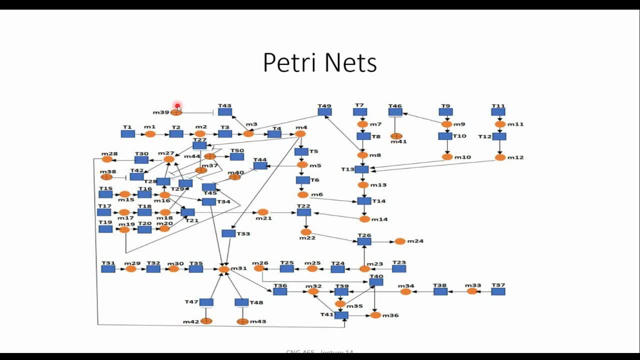 now, when we are dealing with discrete patronets, it means that the places are discrete. they can get natural numbers only. but when you want to deal with mrna or protein levels, then we are not dealing with necessarily natural numbers. so we need continuous places. that's why i can use real numbers. 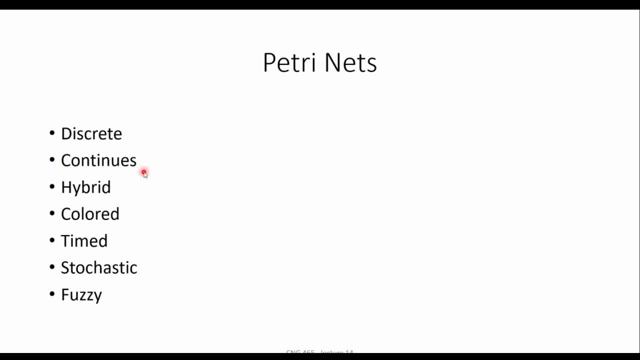 so continuous number, continuous places would be needed, but in some cases, for example for mutation, whether a gene is mutated or not, so this is a discrete case. so you can see that in this case i should consider both discrete and continuous places in the same model. that's why hybrid petnets are useful. when you hear about hybrid petnets, it means that it 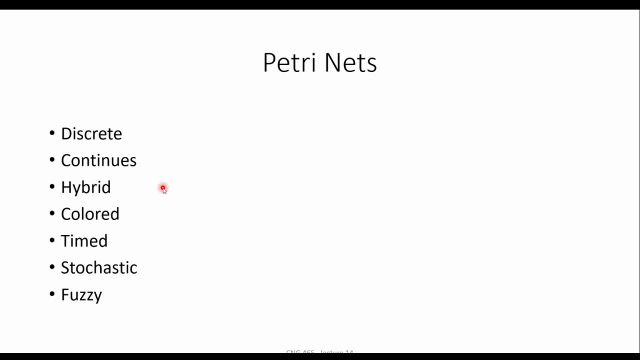 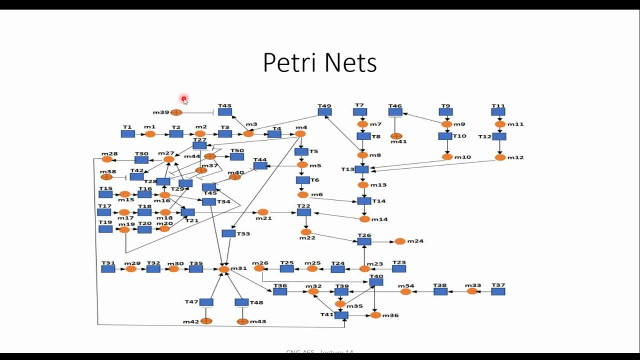 includes both discrete and continuous places. what do we mean by color? inside these places, we can have, as we call them, tokens. so, for example, this is a place. this is a transition. let me show it like this. it's a transition, by the way, transitions can be shown by a line, or rectangular, or square. 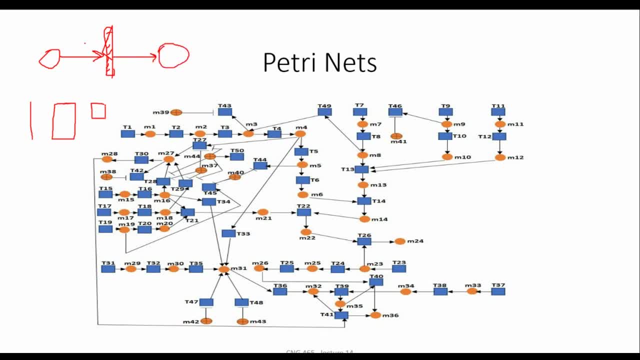 so here, assume that is as simple as i shown in this example, so i can show you how many of that entity i have, for example, three of them. if we are dealing with discrete case, we are dealing with natural numbers, so you can easily show them by dots or you can just 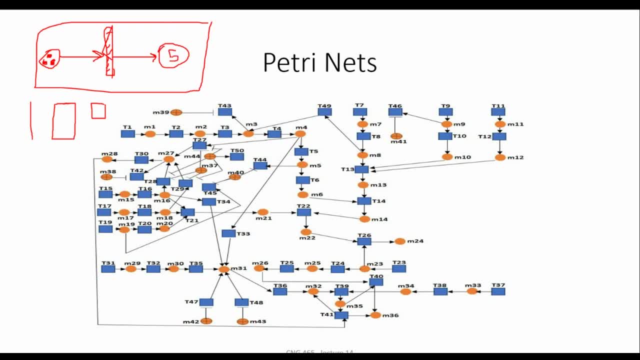 write the numbers inside them, five, for example. it has five tokens now based on the weight of each arc. i understand that this transition can be activated or not. in another word, we call it: does it fire or not? for example, if the weight of this arc is two, then i check in my place that. 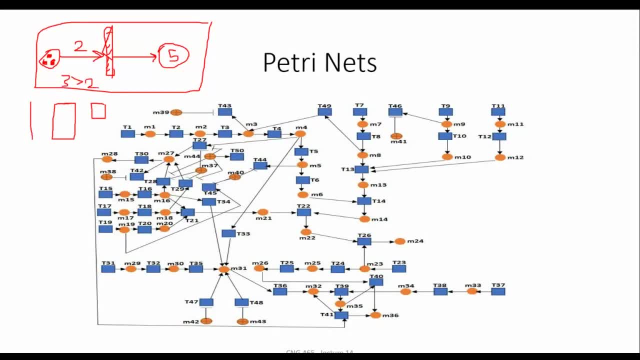 how many tokens i have. three is more than two, so it means that this transition can fire. so what i have after this transition fires. i will have only one token here and i will have seven token here, because it adds two tokens from here to this place. so that's how the classical petronet works, but for continuous one and hybrid ones. 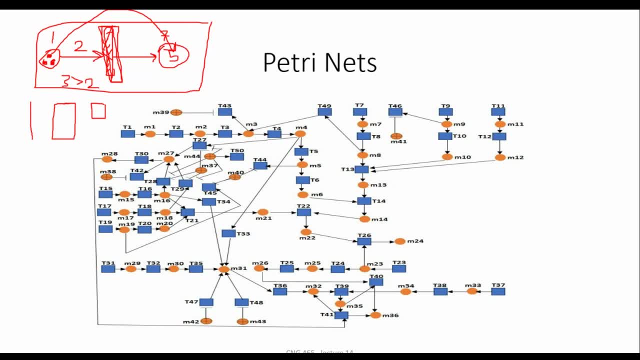 this transition should have a rate and based on this rate we can decide, for example, how many of the tokens will be added to the next one, and so on, and also it's possible to give weights to the arc and define the rate on the transition based on the. 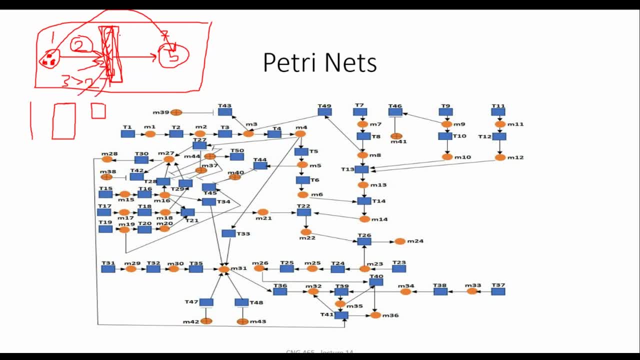 value of this transition. now, if i can do it without changing it. so i can change it to one, and i can change it to one, and even if i don't change it to one, i can change it again. i can change the value of the weight in the next one, and so on. we can see how many tokens we have. 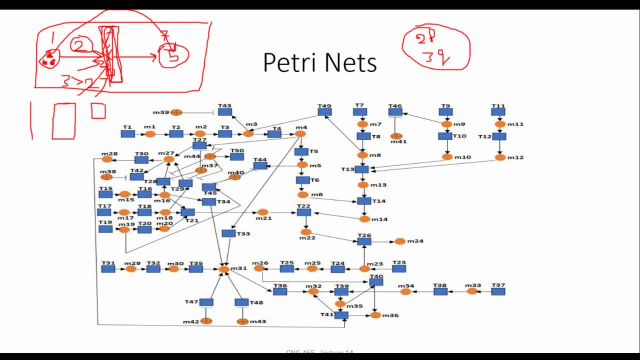 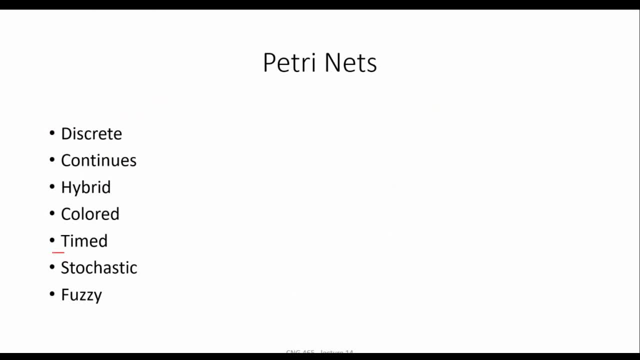 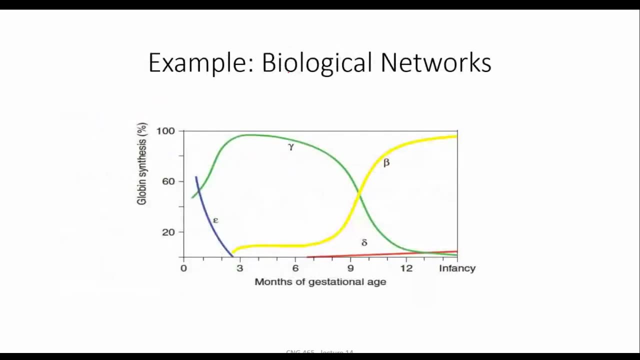 queue, something like that. then this one- we call it a color petnet, because we are using different type of tokens inside these places. time patroness can be also very useful because, like, for example, in this picture, you see after a point we are done regulating one specific gene expression. 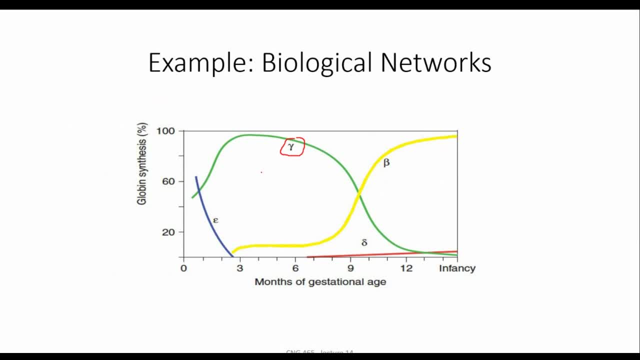 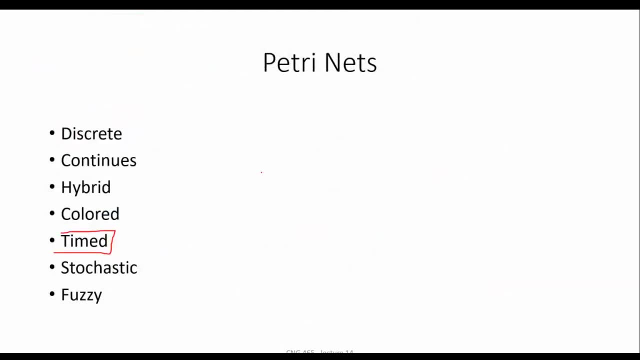 so time uh could be useful, but uh, in my experience i didn't even need them to deal with a hemoglobin switching, for example. it's possible to use hybrid petnet to deal with the time problem by using both discrete and continuous places, because we try to avoid new properties as much. 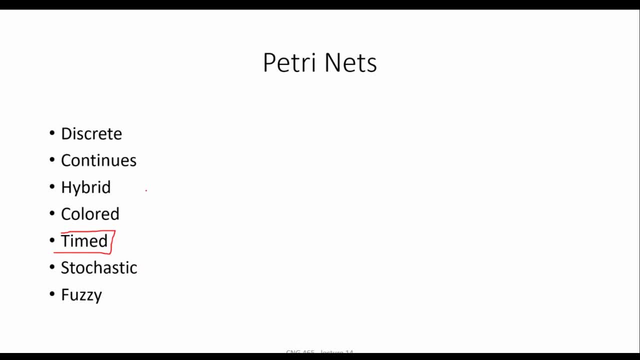 as possible to make our petnets simpler, but whenever it's not possible, whenever we need those properties, then we should add it. so we should know about all of them, and they are not just limited to these properties that i wrote here, and sometimes you hear about extended petroness, extended petnets, 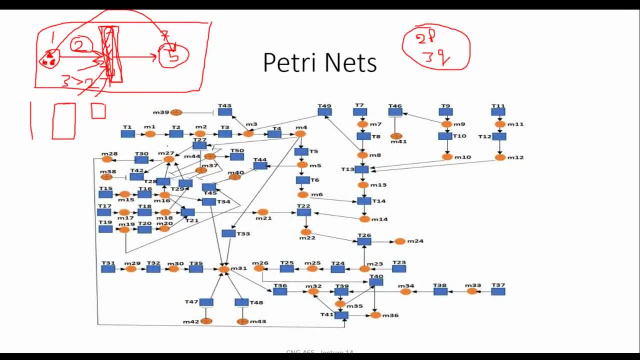 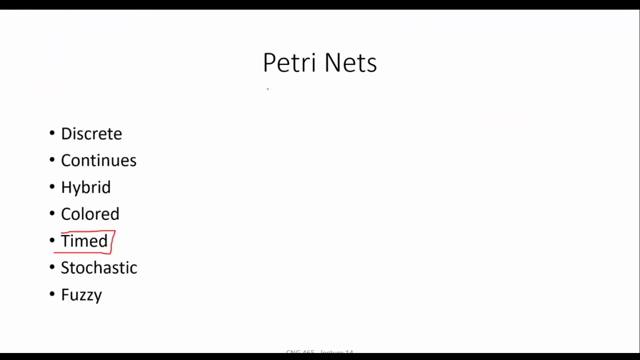 they have also inhibition, like for example here: this is a extended petronet, because we have inhibition as well included. here again, inhibition can be modeled without considering the inhibition arc, but this one is very useful and makes our job much easier, so i myself prefer to use extended. 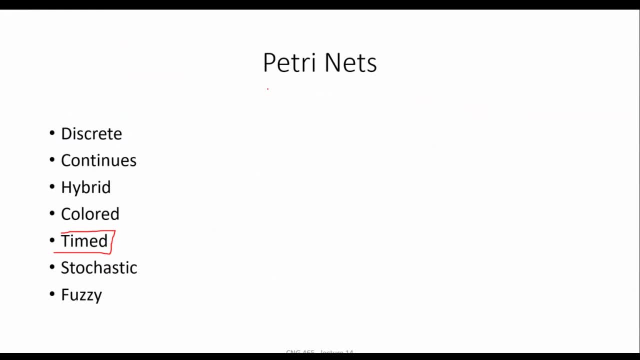 petnets and these days the software. fortunately, they cover mostly inhibition as well. now, these two parts are very important because when you are dealing with biological networks, we should know that these transitions are working in an in a stochastic manner. for all biological networks this is the same story. so if i say, for example, from this place to another, 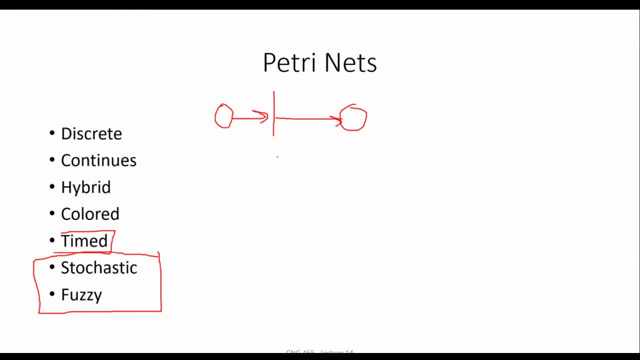 this one will fire uniformly. this is a mistake, and if i have another transition here for another place, then it's not working like, uh, in a linear manner. this one fires and this one fires. in biological system it doesn't work like this. so we should consider the stochastic property. 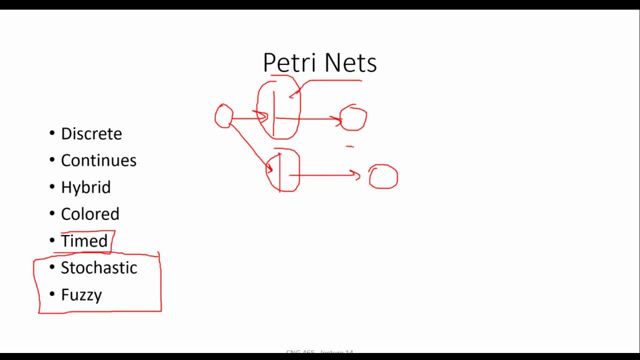 of biological system. so for these transitions, i should consider them as the stochastic transitions. and there is a big reason for it, because when i'm running my simulation i will show you how to run the simulation results. then in that scenario, i need to run so many simulations in. 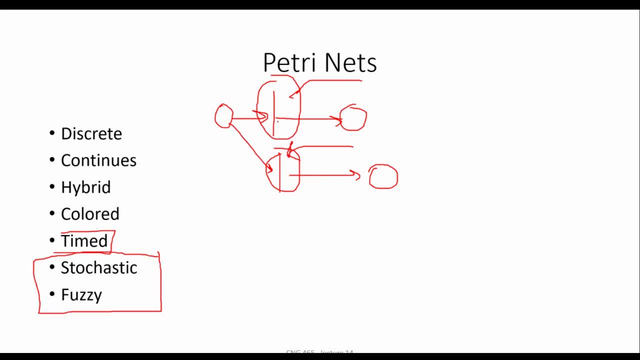 order to get a result. if i consider these transitions as deterministic, just one time simulation, because no matter how many times you try it, you will you will receive the same answer at the end. you will same. you will receive the same simulation result at the end, no matter how many. 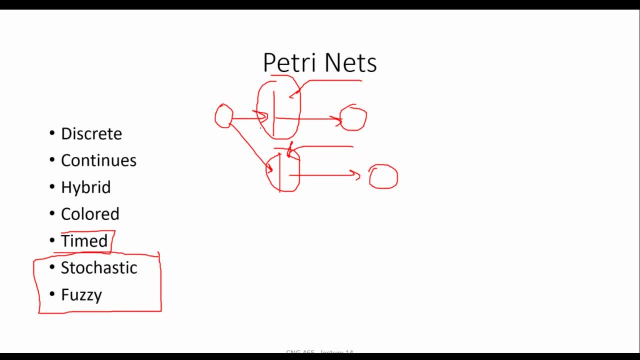 times you run your simulation, so stochastic ones could be very useful. the other thing that we are dealing in biological system is that the rates that you receive for kinetic parameters, these rates that i talk about in transition, we call them kinetic parameters- these ones can be weighed. these 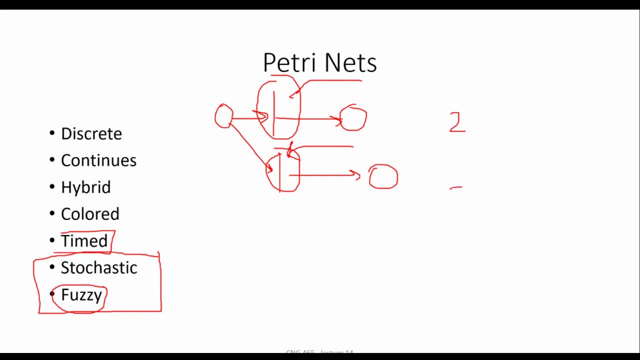 ones are not crisp, as we say in mathematics, like this is not exactly two. this is not exactly two: exactly 3.7. as you remember, in our previous examples, like i told you about grouping genes, then i gave that i've given you information related to gene expressions in different 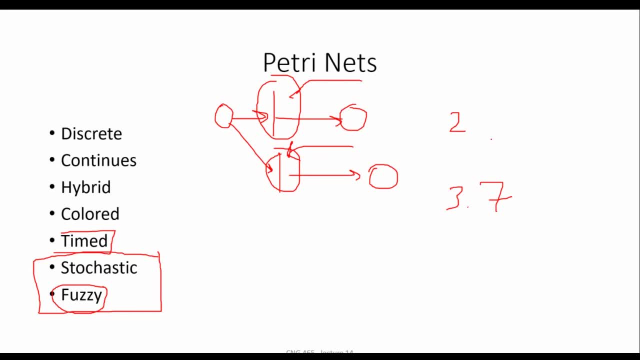 experiments, you observe that in different experiments you don't receive the same gene expression level. so when this is the case, it's not true that in my model i use a crisp number like to say, for example: uh, all, always the transition rate is two, always this is 3.7. this is not correct. and also my places, i don't know how many. 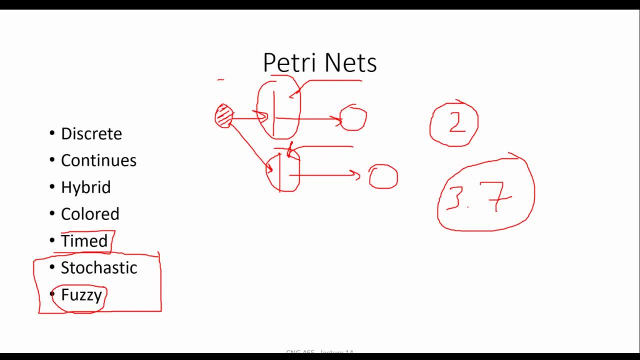 uh, tokens i have exactly in my places. i have exactly five, i have 6.2, i don't know, but i can approximate them. so that's why fuzzy logic can be very useful when you use these models to model biological systems. otherwise you will have huge errors. 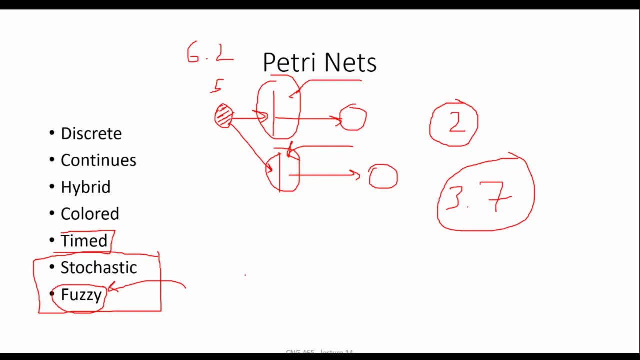 in simulating what's going on in nature. and if you want to know about fuzzy logic, i'm sure most of you guys know. but let me remind you very fast that, for example, for you guys, when i say the weather is warm, the definition of the weather is warm for you guys is different. 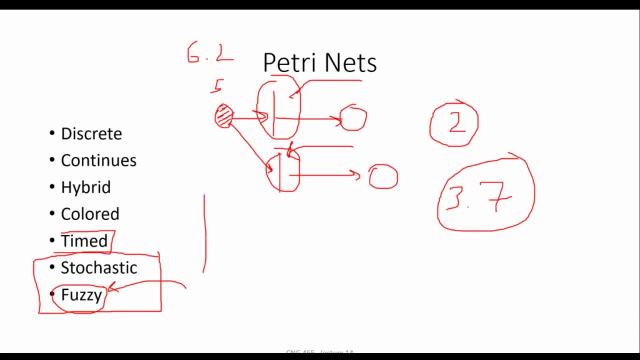 talk about it in weather temperature, like, for example, a person would say starting from 20 degrees centigrade, then I would say the weather is warm. another person says for me, 70 percent, 17 degrees, so this is different from one person to another, so it's not a universal thing to say: at 20 centigrades, then this is: 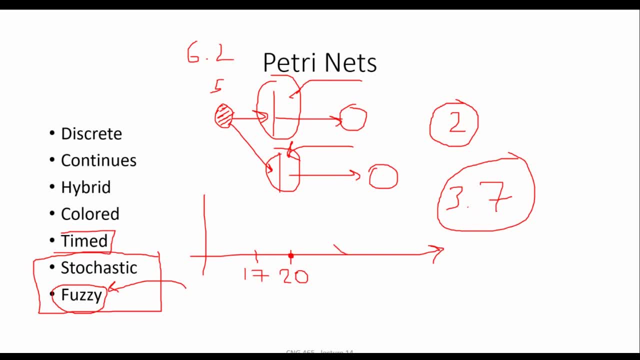 warm. so how do I deal with that then? for fuzzy numbers, they show it with different shapes. the most simplest, the most simple one, is related to triangle. it means that in this format you will have three points, you have a triangle, and in this triangle you will have three numbers: a, B, C. so you can show it as: 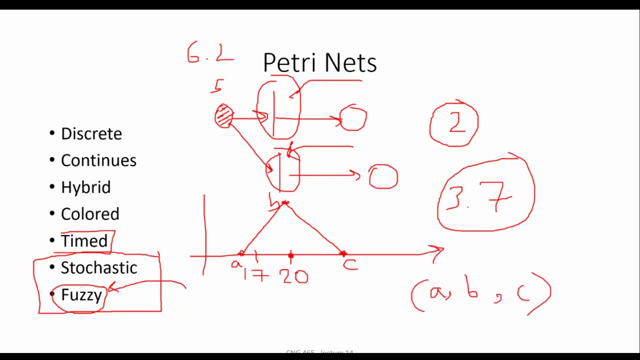 an array as a topo with three components. so a and B shows your boundaries and B is the place with the highest members, as we call. so for each one of these points also, you can have a single bar in your field. you can have a single bar in the. 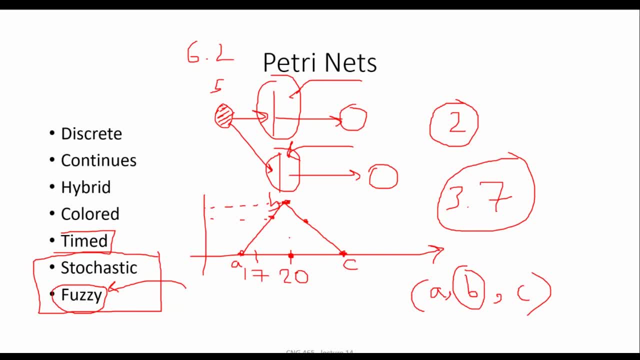 other, and every single bar is with the highest number and every number is with different memberships here. this is the way we can deal with that, so when someone else is talking about, for example, cold weather, you can have another fuzzy number for that. by the way, it should stop here at the same point. 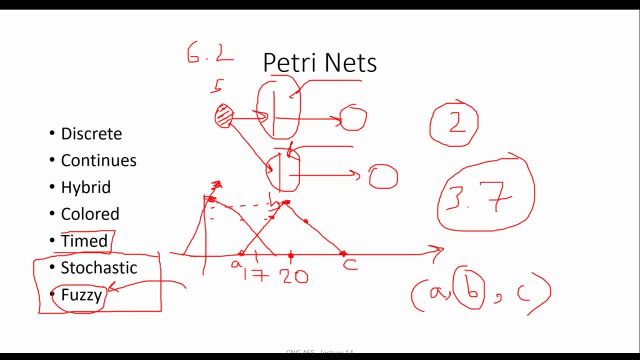 yes, then you will have two different fuzzy numbers. this line should match here because they have the same membership one. okay, now you can see that here we have even intersection between them. the weather that you consider warm is considered cold for some people. so you see, fuzzy numbers can be very useful. 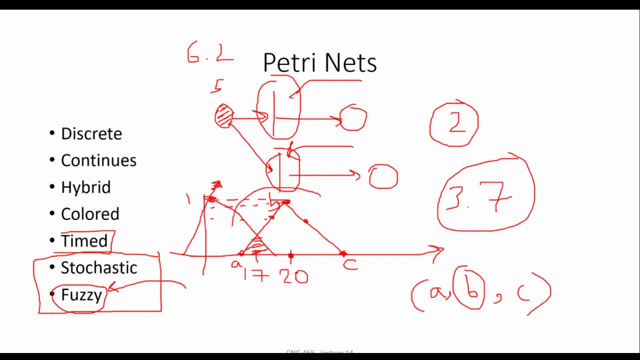 also for biological systems, because now we can deal with an interval and each one of these numbers can be used for biological systems, because now we can deal with an interval and each one of these points, they can have a membership function. to be more sure, for example, this is the value that you are looking for when we are talking about just a. 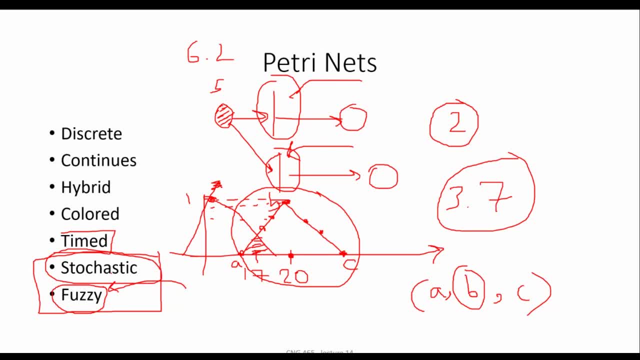 stochastic biological system or stochastic models, then we are dealing only with this number B. that's it. we don't consider the rest of it. so instead of just saying starting from 20, the weather is warm, I can give a fuzzy number for that. so that's the logic behind it. 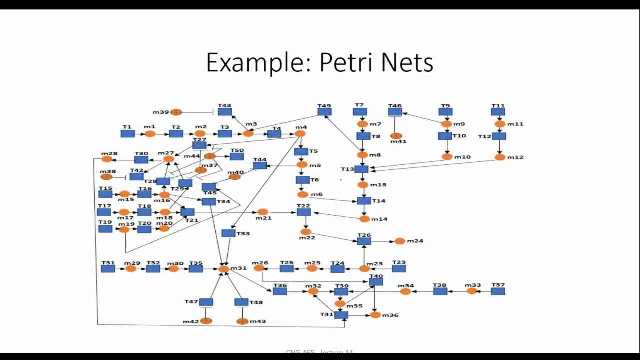 so that's the logic for using fuzzy numbers for our places and also for transition rates. you can do the same. so at the end, when you receive the simulation result, you will receive the fuzzy numbers. so, as you can see, the picture is exactly the same as the previous one I shown you here to know. 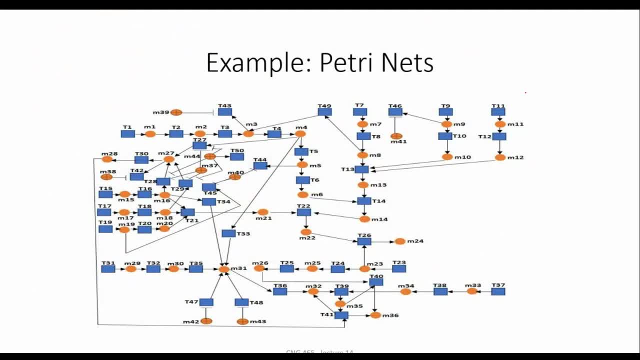 that this is a stochastic, or this one consider, for example, fuzzy as the property inside it- then we need to give you tables, we need to say, for example, these transitions are defined as stochastic transitions, and so on. so it will get even more complicated, but for you guys, it's just good enough to know. 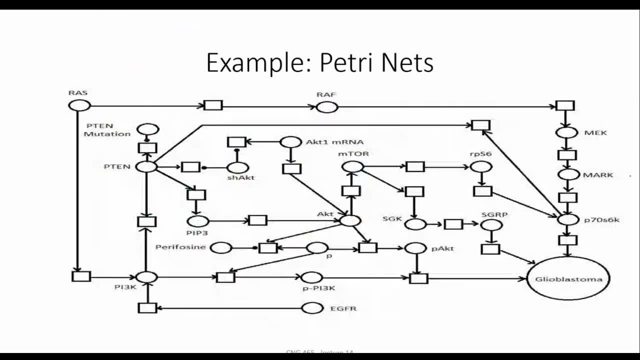 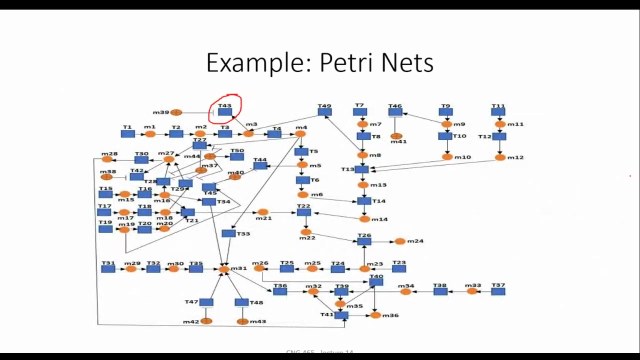 that we have different types of computational models and that's how we can deal with simulating biological networks and personally I believe that when you consider hybrid and also stochastic and fuzzy, and even considering extended pertinence, you can cover most of the biological networks and you can easily validate them. for example, I use the previous one for beta. 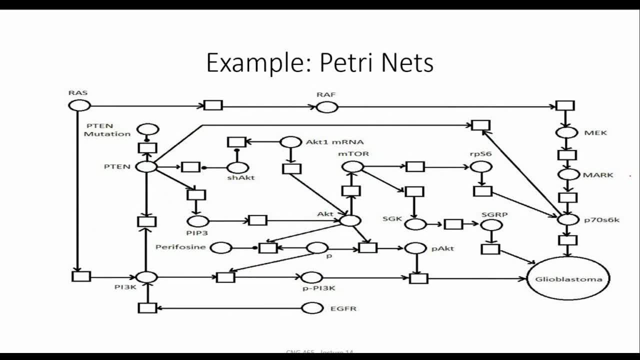 globin and I use this one for brain tumor and neural networks, and this is it in my case. it's very sophisticated. so if you ask me, for example, how do I choose, for example, which pathway? so again you should go to that website cake, and you find a pathway. does cake contain all the components, as I say at the beginning of? 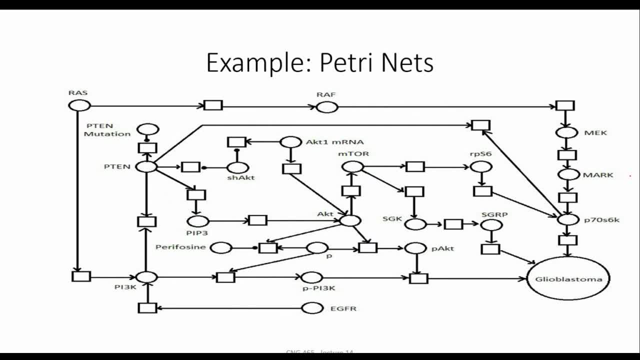 the session that this is not the case. you should read different articles in order to know, for example, even just this little transition rate. that's it for articles. to know, for example, which transition rate i should use this one, and even to consider it as a fuzzy number. it takes time. so, as you can see, these topics are very complicated and 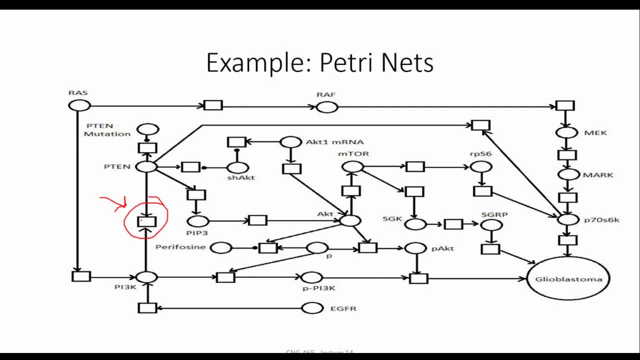 we usually talk about them in advanced bioinformatics. but for you guys, i think it was interesting to at least get ideas that what's going on. and for those who are interested to be bioinformaticians, or at least when you consider continuing your education in computer science, then 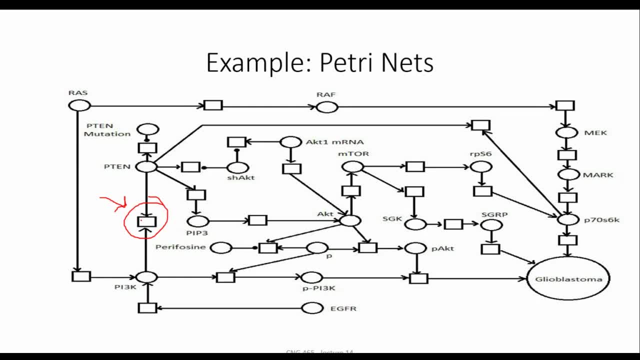 this could be a minor for you to consider and take bio bioinformatics related courses which are very interesting, but you should really love this course. otherwise, if you are not interested that much, then it could be very complicated for you, as i mentioned in the beginning of the course that 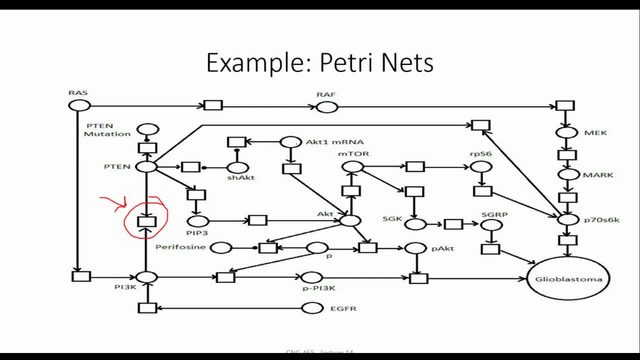 it contains so many topics inside it- statistics, computer science, mathematics, biology- so it takes time. but if you are really interested, because this topic is really interesting, then it could be very useful for you. so my goal in this course was to introduce you about topics related to bioinformatics. 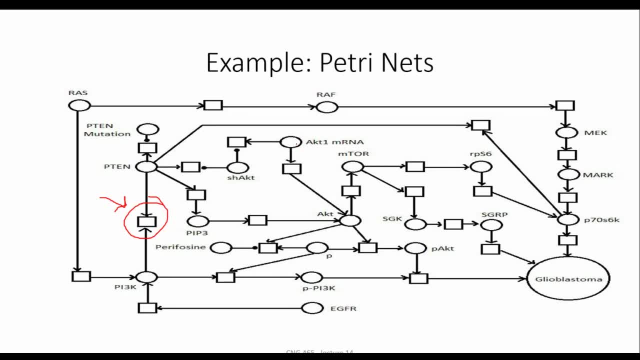 and i hope you got the idea that what's going on. but in the exam of course we are trying everything manually uh, but you can practice it after the semester just to try, uh, the examples that we have and try to write programs for them, to practice that how you can deal with them. it could. 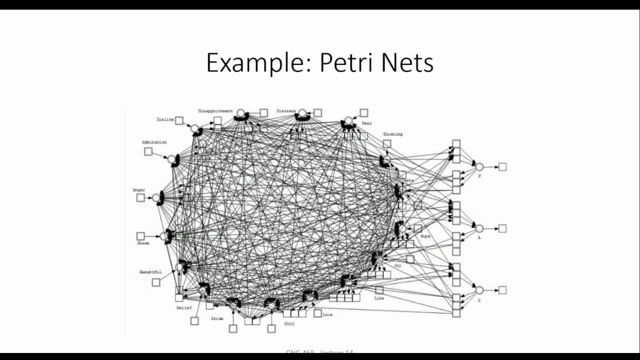 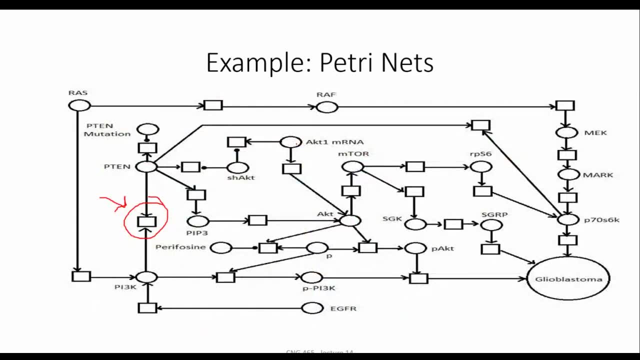 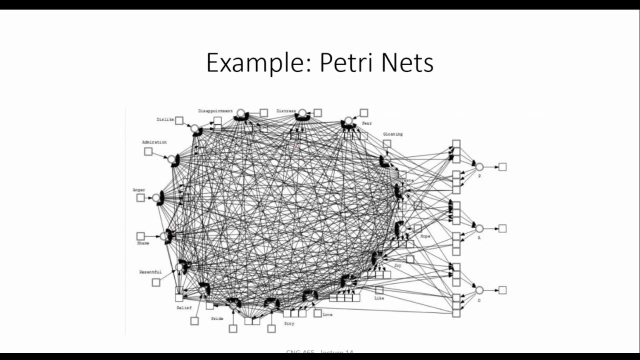 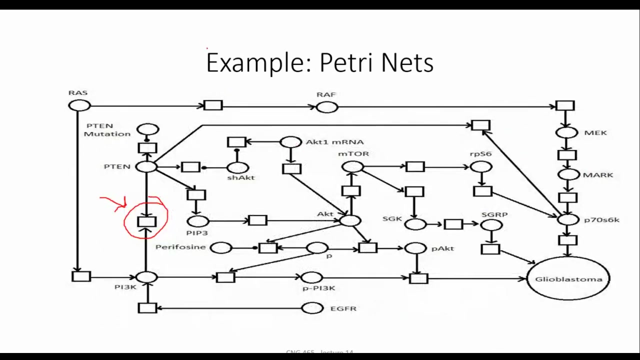 be interesting. okay, so i mentioned about two examples of beta globe and brain tumor and for example, for psychological тобias, for psychological systems. we can do the same even for biological systems. we can sometimes have such complicated patterns so it's not as easy to say there is one arc from one place to another and so 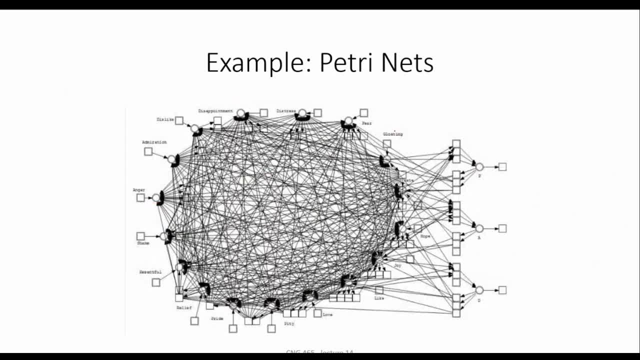 on. it can be complicated. so here, for example, i try to simulate mood based on emotions. so our emotions are interacting with each other and all the components are interacting with each other. so again, to understand each one of these rates, we should, for example, study very much to understand. 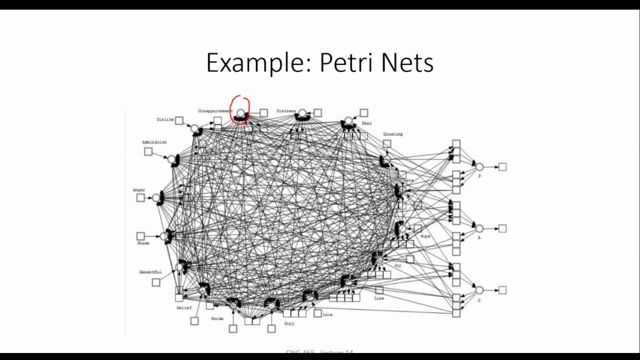 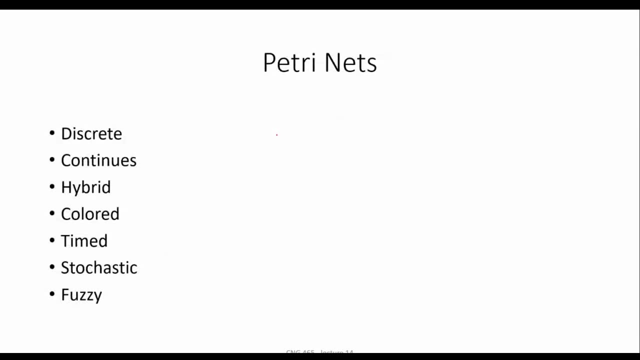 what's going on between each one of them. so, as you can see, these things could be very complicated and if you are really interested in these topics, we really need bioinformaticians, more bioinformaticians, to deal with that and hopefully some of you will be interested in this topic. so, again, to sum up, we have we had different types of 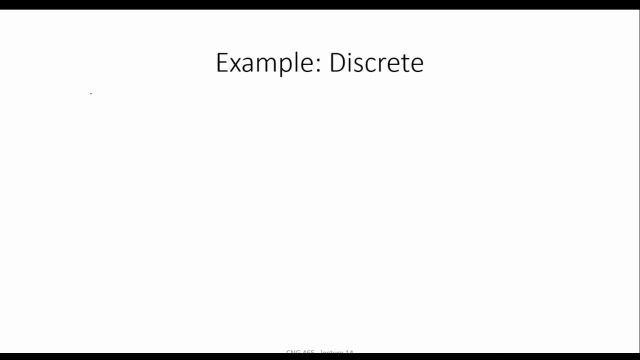 patronets, and i can also give you some rough examples, like again for the classical petronet. let's say we are talking about hydrogen and oxygen, oxygen and you have water here. so here i should specify, for example, if you have two hydrogen molecule and one oxygen. 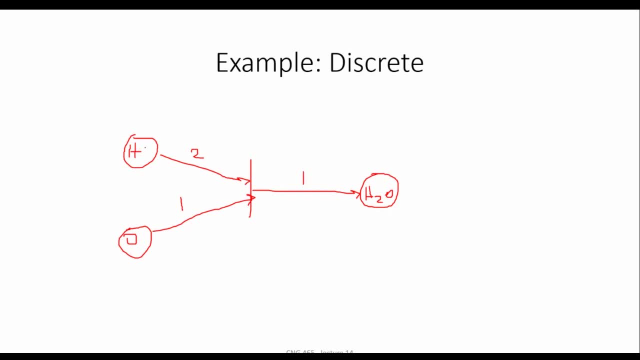 then you will have one water. so this is the way it works. so, based on the available tokens in them, you can have water molecules as much as tokens we have. and for hybrid we have both continuous and discrete places like, for example, let's say, this place is for mutation. 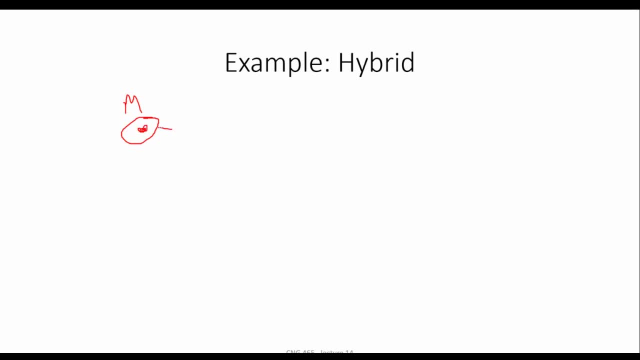 and whenever i put a token here, i can inhibit a specific transition, like for example, for a beta globin, for beta thalassemia. we have this problem. actually, beta globin is down regulated by mutation, because we have this mutation in a particular chunk and a function that we call a mutation. 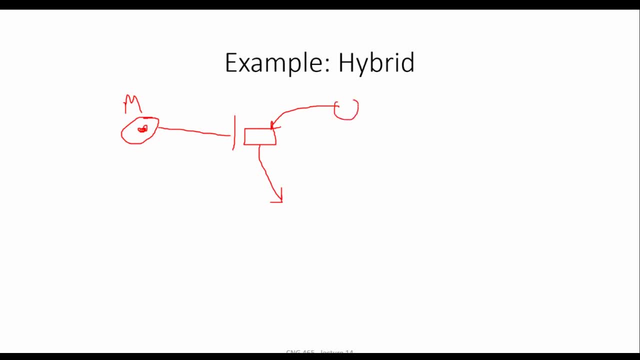 and this transition won't be activated anymore or can't be fired, as we say in patroness. so there are maybe several places here and this mutation inhibits this, a specific square. but the thing is that is it down regulated totally? i mean, does it knock down the gene expression totally? this is also another challenge. so 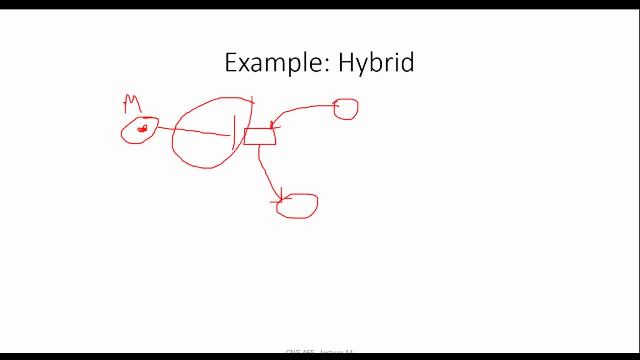 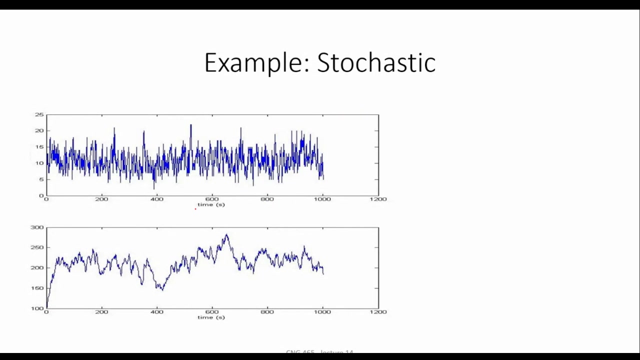 challenge. so not always this is a good idea to show mutations by inhibitions like this, because this inhibition would avoid any firing from this transition. so this is also another challenge we are dealing with, but in my articles I also mentioned how we can deal with that and when we talk about a stochastic. 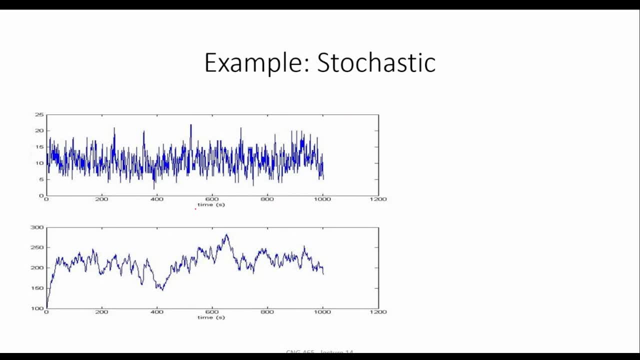 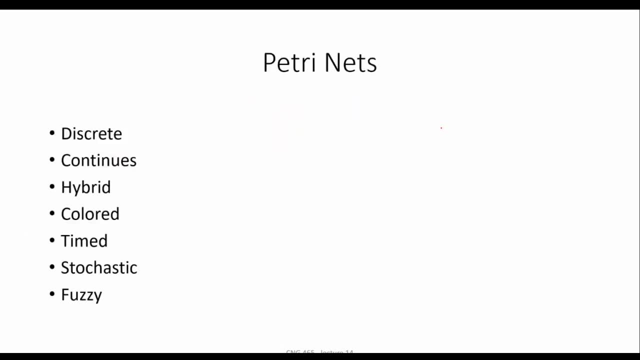 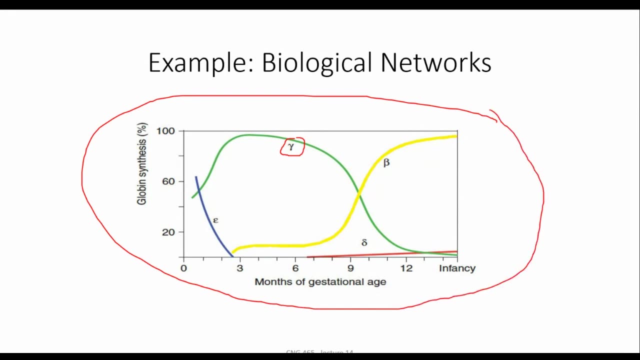 patternets. so for our simulation results, you will see that this is such a mess here. this is such a mess because if I want to reach a simulation result like this in hemoglobin switching, because for deterministic models easily I can reach this one, but when we talk about a stochastic one, it sounds like such a. 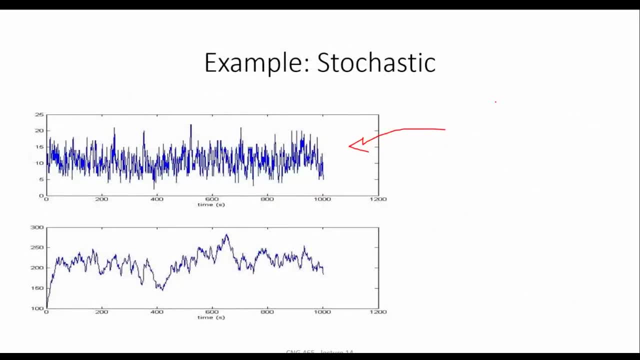 mess, but how do we deal with that? we have so many simulation runs, so we get the average of them and you will find a better trend like this and you get ideas that what's going on here and we are interested to reach a steady level. it means that, if I 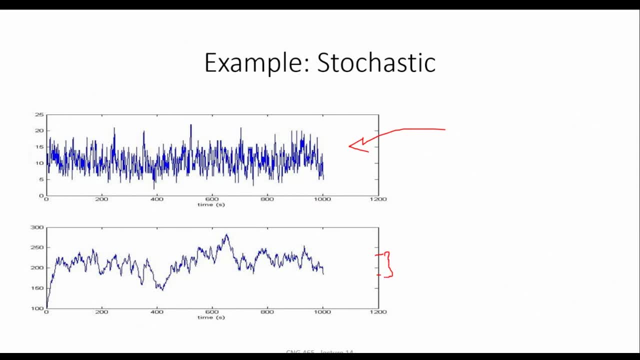 consider a neighborhood like this. I should from, for example, this point thousand. my simulation should show the trend between this interval. if I reach that, this is a steady level and usually come 2. scientists are very interested in a steady level because of this, because if you reach that, no matter how many simulations you will have in 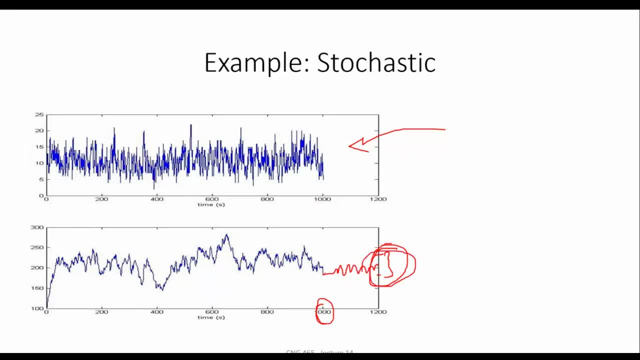 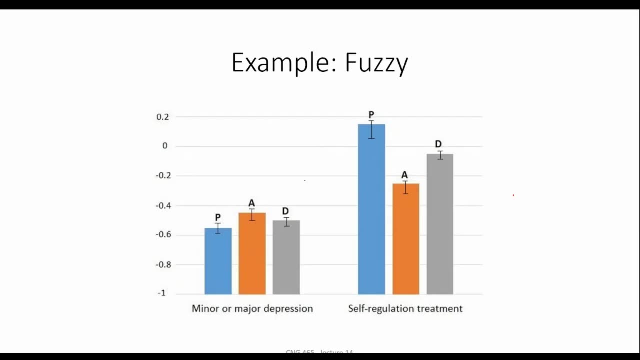 your model, then it should be in this interval. if you reach that, it means that you reach the steady level and you can report your simulation result. and that's a beauty of a stochastic patternets, because we are not only dealing with a deterministic one. it is not played on the equation in this example, but it is a test of whether you really outperformed or not what you did in the two things that you done. and the problem is if belief means to work and right to that agents. one and the other problems does not solve and relates to a manipulation- almost the same thing. but we tellkaa that this is our most of the以上 to not getting that information right now. if you say we didn't get positive, 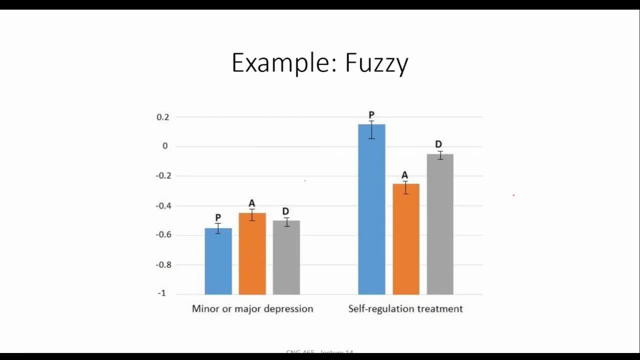 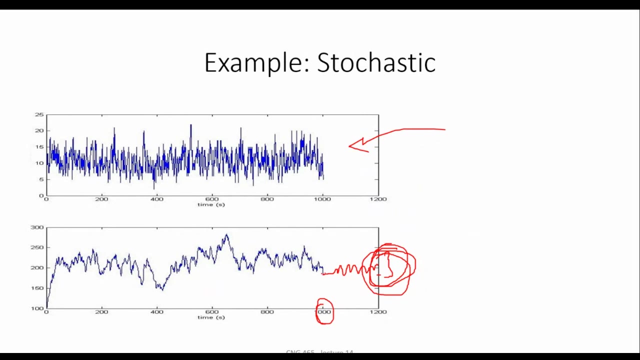 that has only one simulation which has most probably high errors. and when we talk about fuzzy simulations, as you can see now, we are dealing with fuzzy numbers, not just the point, because if i want to report my result here, i would say, okay, what's the point here? 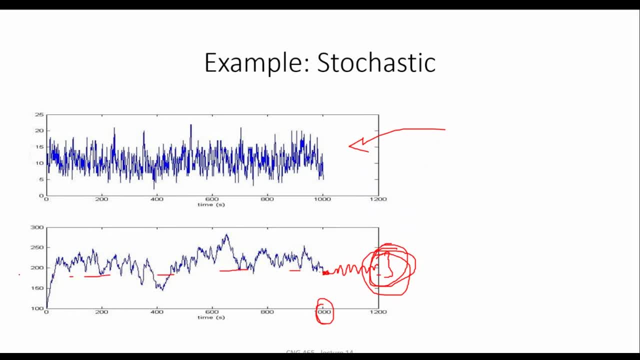 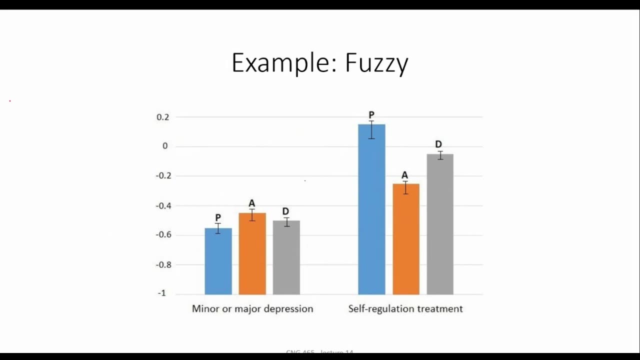 for thousand, it says, for example, 185.. so i will report this one as the simulation result. but for fuzzy numbers i should report an interval, and these points, as you can see here, for example, this one is exactly the point that you report for the stochastic one, and these points are the boundary points. 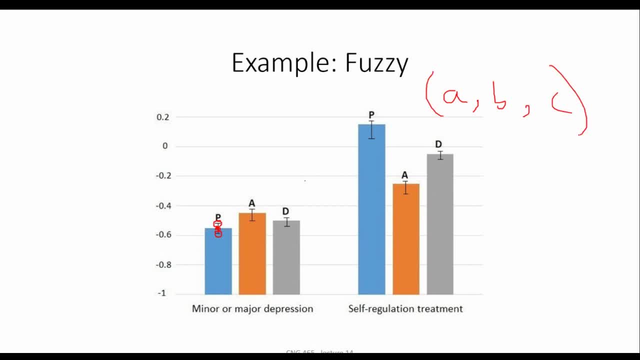 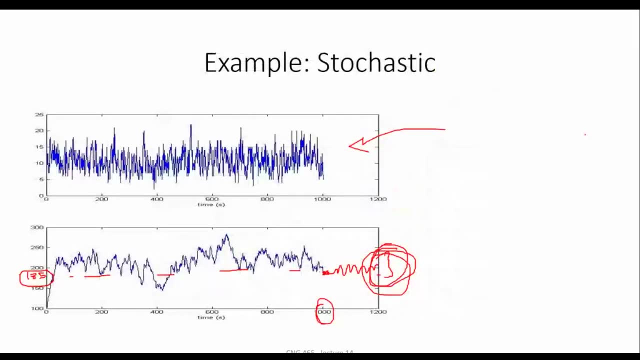 so there are a, b, c. if you are interested, of course, you can read my articles in google, scholar and researchgate to know more about it. and for a stochastic one, i also have an? uh. i have a video related to stochastic processes. uh, in a stochastic course, if you haven't uh taken this uh a statistic course from: